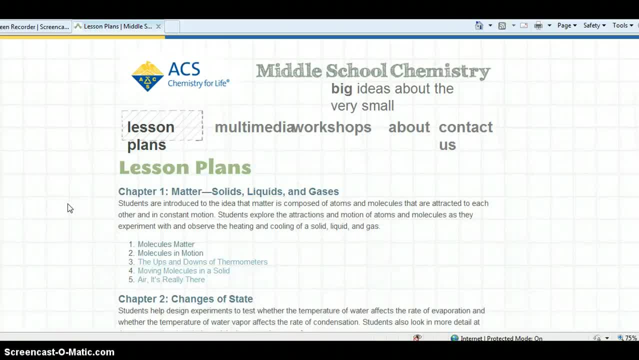 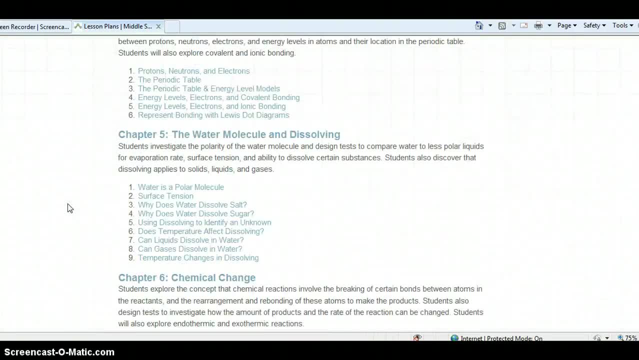 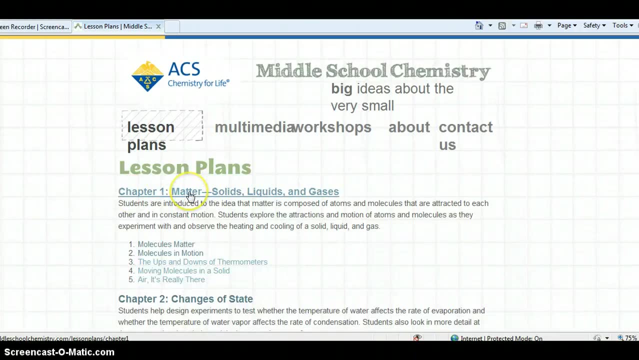 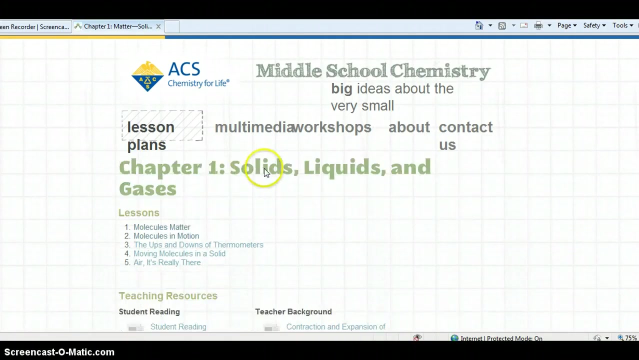 and really try to understand what they're learning or if they need extra help. It has many different lesson plans listed here that go in order of least difficult to most difficult. First we're going to click on: We're going to click on this chapter one, and this is just the overall unit, which is solids, liquids and gases. 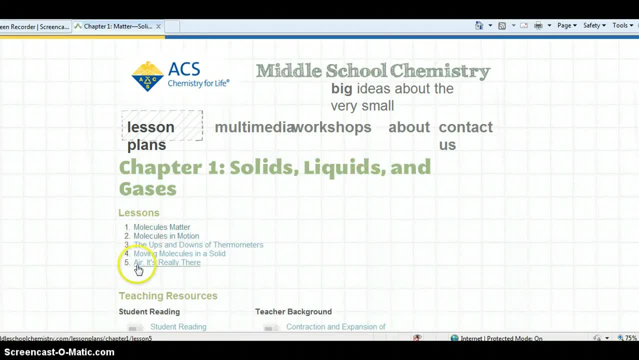 And then it has different specific lessons within the unit. So we'll take a look at molecules in motion here, which would be the second lesson within the entire unit. As we scroll down here, we can see what the lesson is made up of. 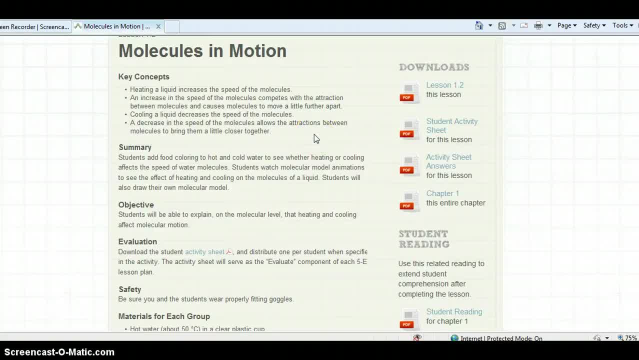 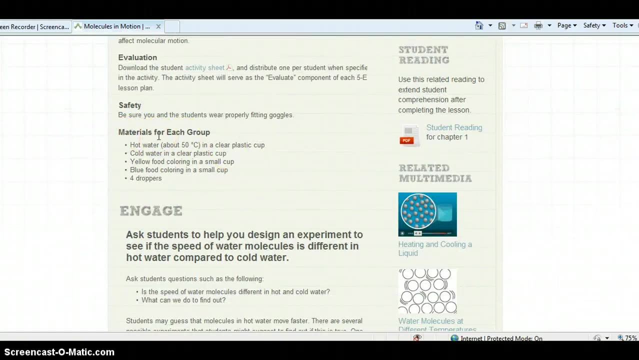 It shows the key concepts that your students will learn, or hopefully learn, with this lesson: The summary. The summary, the objective of what you would like them to learn, an evaluation and safety precaution. And then it also shows different materials that will be needed for the experiments or whatever this lesson calls for. 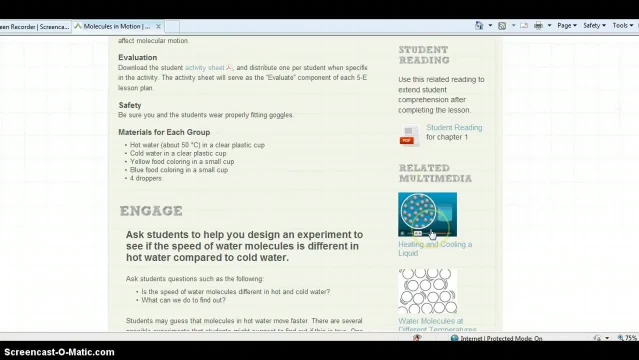 Over here. it has related media, which is different types of video, audio visual aids that could help your more visual learners get a greater understanding of the material that they're learning in the lesson, or just a another way for everybody to understand and really grasp what you're trying to teach. 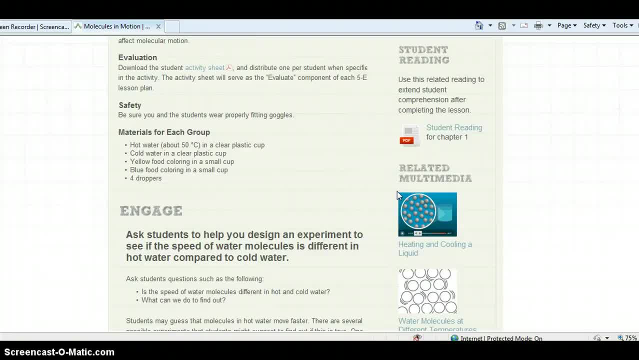 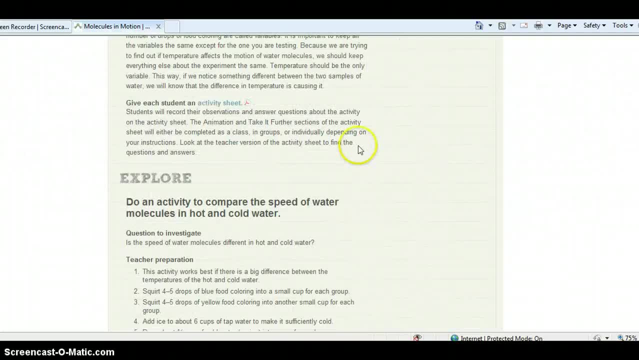 I think that these lessons, like I said, could be especially helpful for the new teachers, but also for the experienced teachers, being that they have such great detail. It really goes through here different things to explore how to get your students engaged. 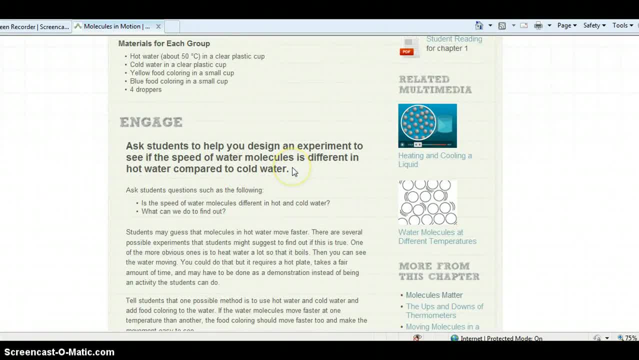 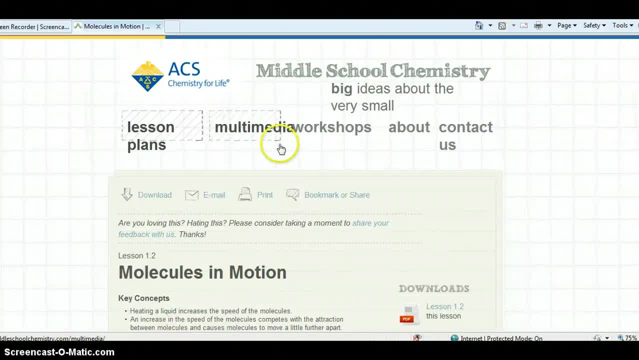 I just really think that this is a great tool to use. I just really think that this is a great tool to use in the classroom and also for students. I just really think that this is a great tool to use in the classroom and also for students. 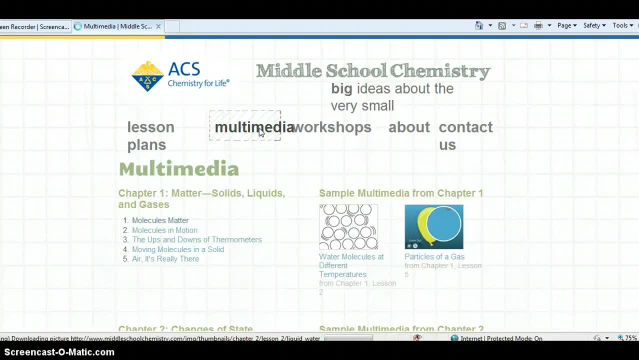 Then if we go to the multimedia part of this website, it gives all of the different types of videos and visual demonstrations of what exactly they're supposed to be learning. I think especially in chemistry this is helpful because it's a very abstract kind of content that they're trying to learn.